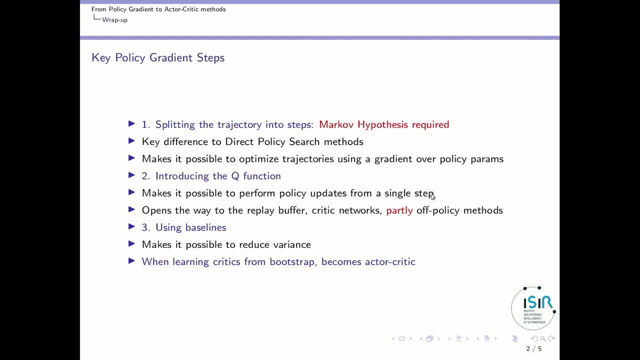 from policy gradient methods to actor-critic methods. okay, Because it opens the way to using a replay buffer, to using critic networks and to move to off-policy methods. But, as I will insist on on the next slide, those methods can only set partly off-policy. The third key step consisted 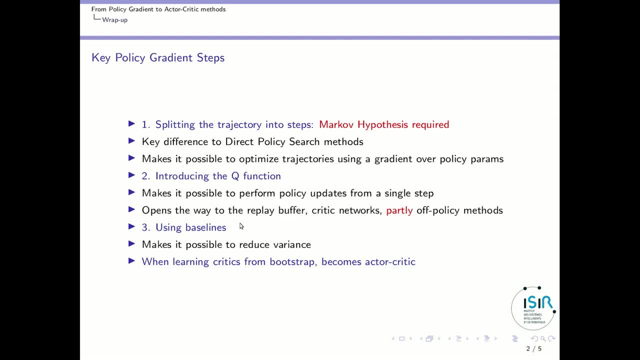 in introducing baselines. Using those baselines, we can set the policy updates from a single step. The baseline makes it possible to reduce the variance. but, most importantly, when those baselines are critics and when those critics are learned with bootstrap methods, they become actor-critic. 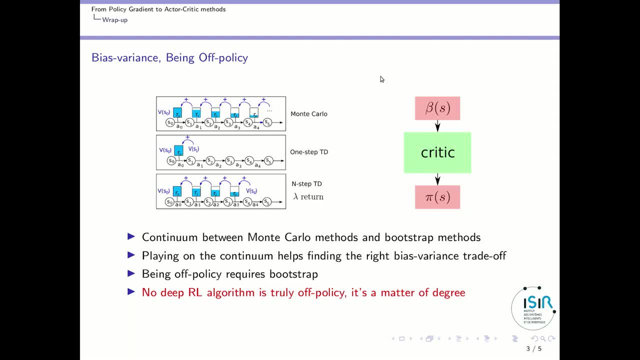 The second thing that I want you to remember about those lessons is about the bias-variance trade-off and about being on policy. So, about the bias-variance trade-off, I told you that you can estimate a critique using a Monte Carlo method or a one-step temporal difference. 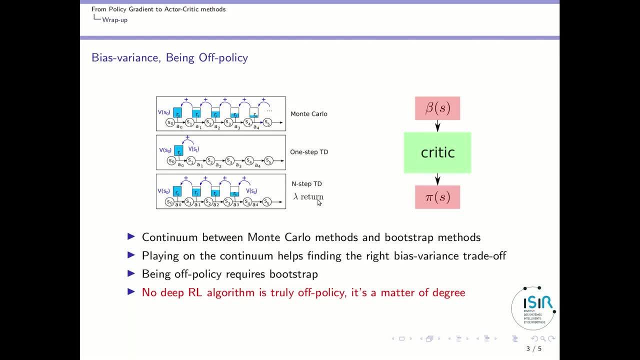 method And that using n-step return or lambda return provides you with something which is intermediate, which allows you to play with a bias-variance trade-off and to find some optimal way of performing. The other point was about being off-policy. I told you that to consider being 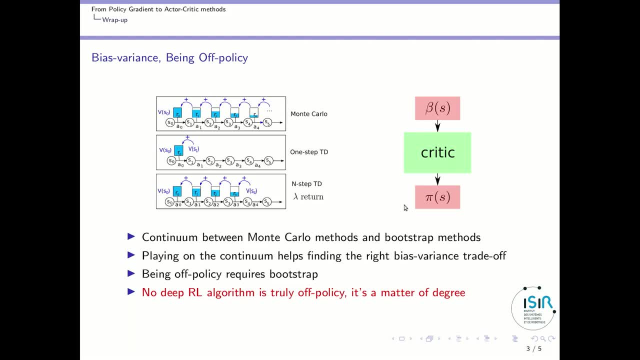 off-policy. you have to distinguish between a behavior policy and the target policy that you are learning, And that being off-policy requires bootstrap. Most importantly, no deep reinforcement learning algorithm is truly off-policy. It means that no deep reinforcement learning algorithm can work from uniform sampling. It's just a matter. 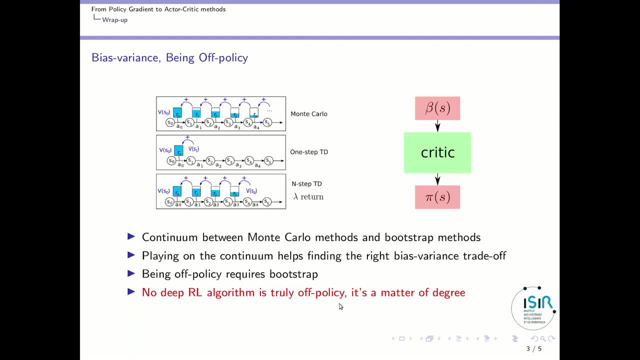 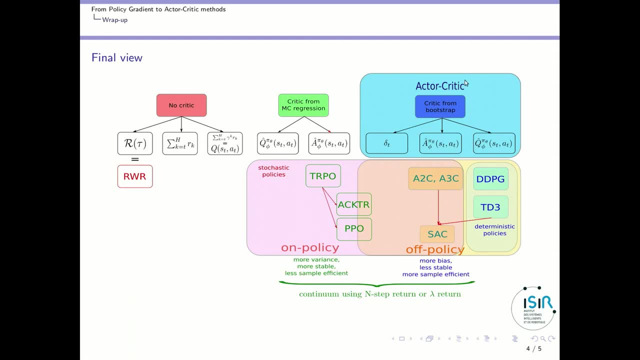 of degree. Some algorithms are more off-policy than others. The final point that I want you to remember is this global picture, where you have here different policy gradient techniques. Some of them use no critique, so they can take just the sum of overrides. 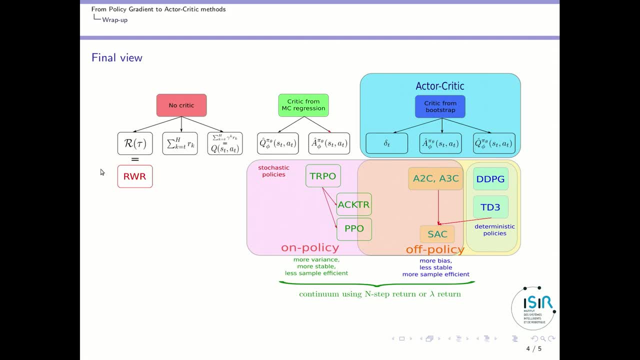 You can take the rewards over a trajectory, And in that case I have shown you that the equation is similar to the one of reward-weighted regression. Or you can take a discounted sum of reward or using a Q function. Another approach is to use a critique, using Monte Carlo regression And this critique.